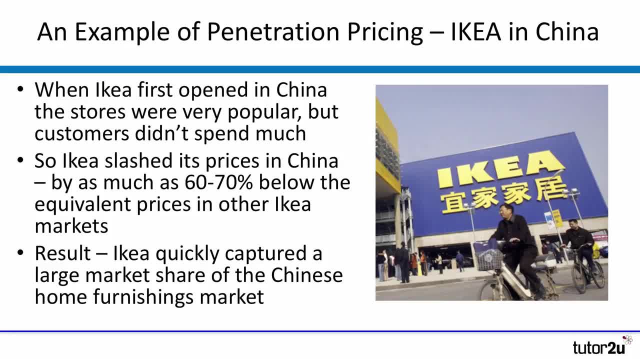 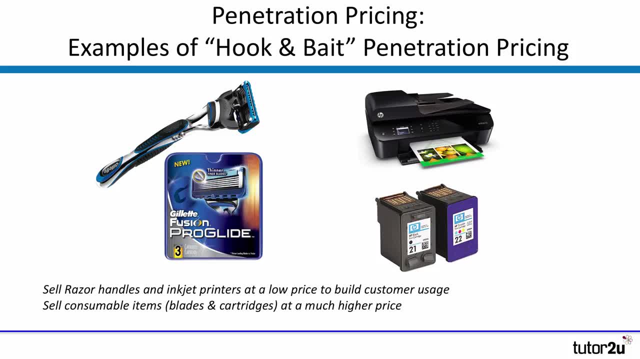 changes to the marketing mix And, as a result, they very quickly became the dominant home furnishings retail player in China. So another example of penetration pricing that you may have fallen victim to- I certainly have. It's what's known as hook and bait penetration pricing, A method of this pricing strategy in 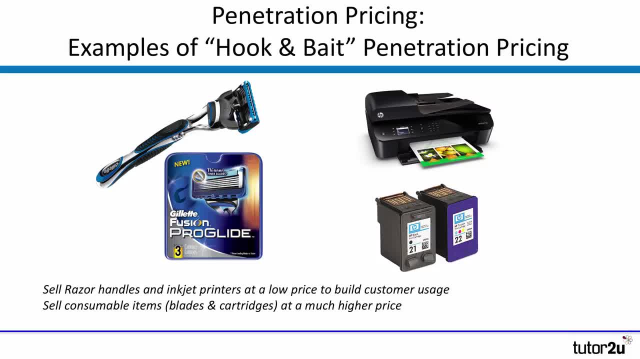 action. If you've ever bought, for example, an inkjet printer from the likes of HP, You often find that the cost of the printer itself is very low. But if you've ever bought an inkjet printer from the likes of HP, You often find that the cost of the printer itself is very low. 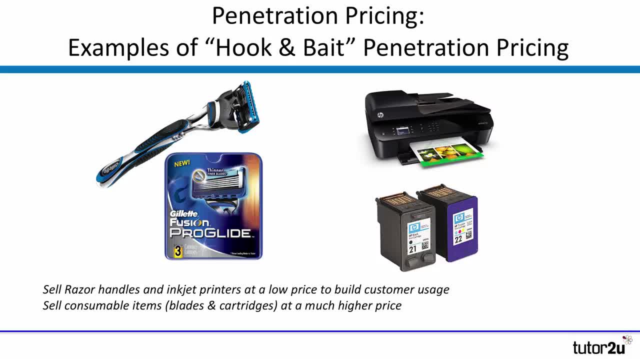 It's only when you start buying the cartridges, Once the initial supply of cartridge has run out, You realize that the total cost of ownership can be a lot higher than the initial price of the printer. So the idea in the same way, The same strategy is used by razor blade, Both for the men. 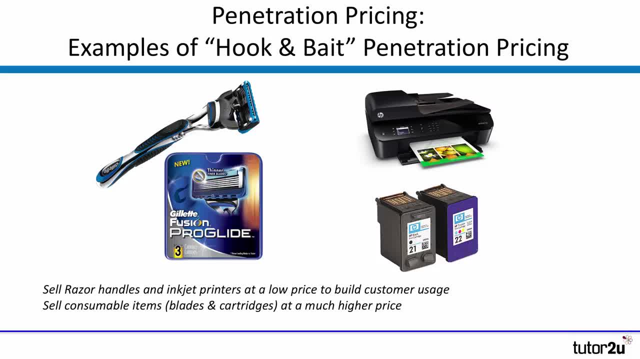 and the ladies, of course. Razor blade businesses sell the handles really cheaply to get people using the handle, But then sell the replacement blades at quite a high price. And that's what I'm going to show you in this video. I'm going to show you how to build up that customer loyalty. 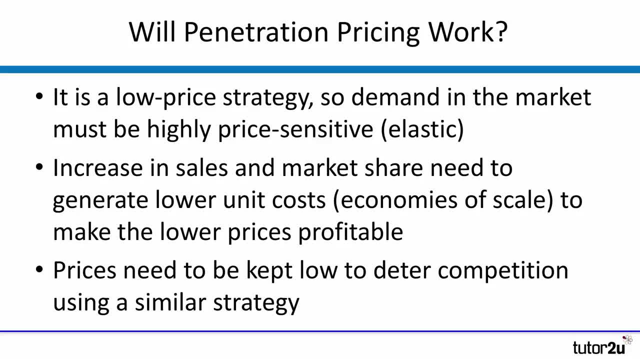 Once you've built up that customer share, Well will penetration pricing work? It's widely used But of course it is dependent on demand for your product being price sensitive. It needs to be highly sensitive to price So that consumers are prepared to switch from existing brands to the 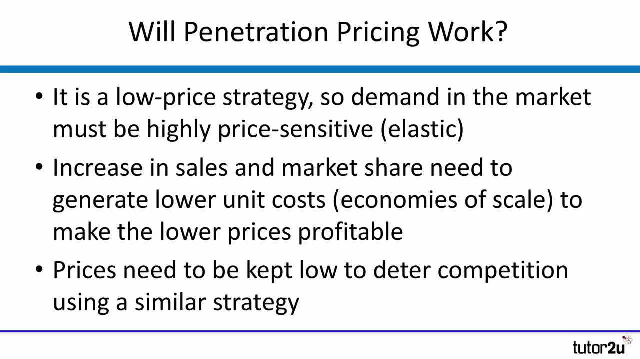 lower priced product, And also you need to be operating in a market, An industry where it will be worth your while to offer an inkjet printer, And that's what I'm going to show you in this video. As a result of doing so, can you achieve the kind of sales that enable you to achieve? 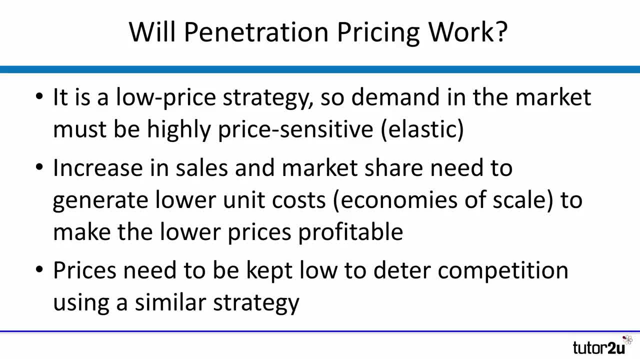 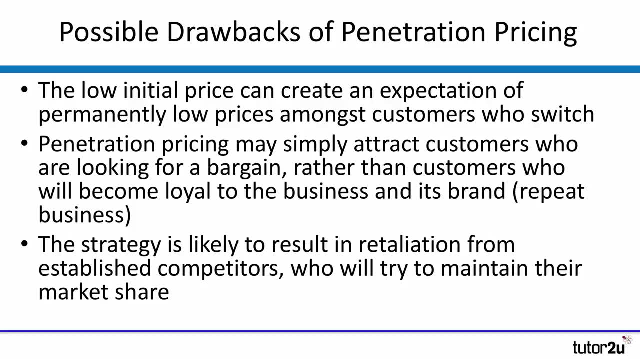 economies of scale in order to make this lower price profitable, And also are you able to keep that price low consistently in order to deter competitors from using exactly the same strategy? You can see from that that there are one or two drawbacks of penetration pricing as a pricing strategy. Firstly, of course, over time there may well be an expectation created amongst